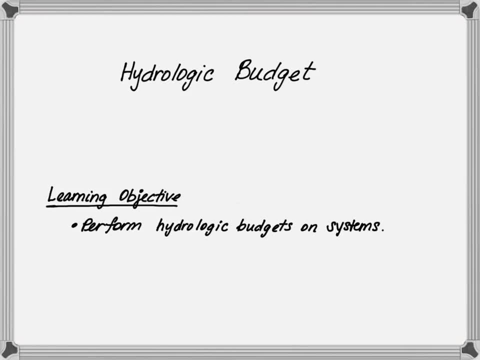 a lake, reservoir, dam, segments of a river stream, canal, roadway and many other things You must be wondering. so what is a hydrologic budget? You could think of it similar to a bank account: We deposit money in, we take money out and we have. 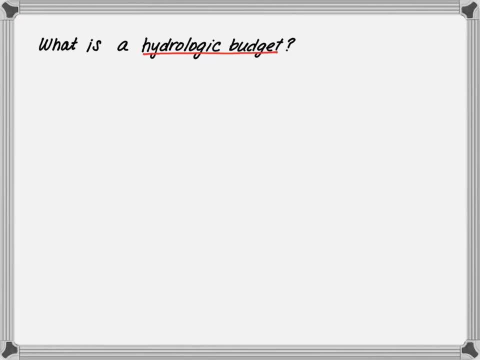 money stored or saved in our account. So a hydrologic budget is similar. Instead of the system being our bank account, it's a hydrologic system. All hydrologic systems are comprised of components of the hydrologic cycle. Remember a hydrologic? 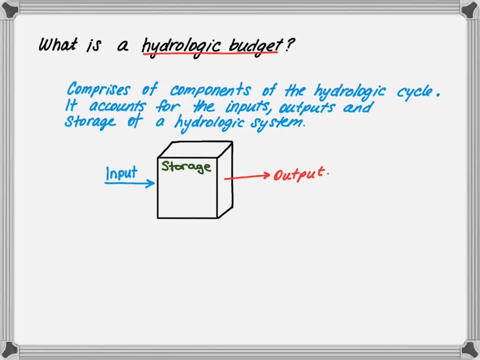 cycle is composed of precipitation, evaporation, transpiration, infiltration, various types of surface and subsurface runoff and storage. It accounts for the inputs, outputs and storage of a hydrologic system, as shown in this example. For example, the following are some types of inputs, Please: 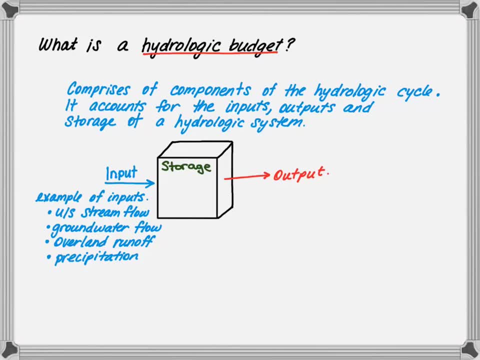 note that this is not. this is just some of the possible inputs and is not an inclusive list. Upstream flow: this is the flow entering the system directly through a river. Groundwater flow, defined as through flow, where groundwater enters the storage due to the subsurface water level being higher than the surface water. 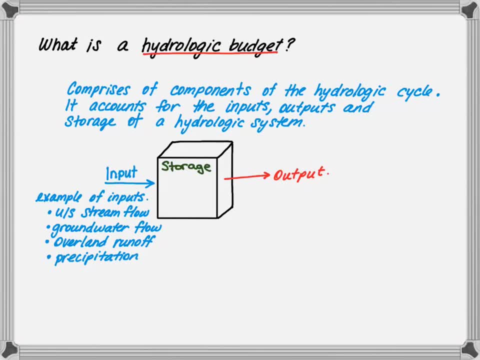 level Overland runoff. this is the water that comes into the system through the perimeter of the control volume, And precipitation, which enters directly into the control volume. Some examples of outputs include: downstream flow- this is the flow exiting the system directly through a river. Groundwater- this is the water exiting the system through 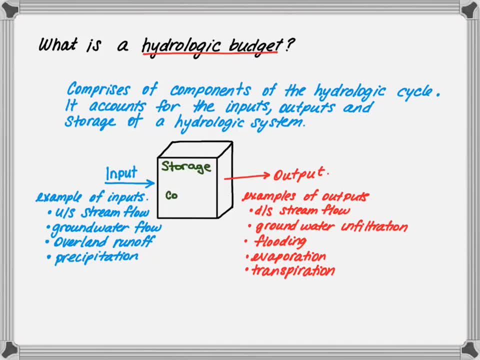 infiltration: Flooding water leaving the perimeter of the system, Evaporation flows evaporating from the surface of the system And transpiration flows evaporating from vegetation within the system. And finally, the storage is the control volume of the system. 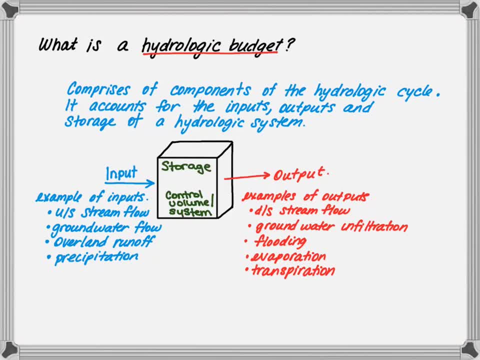 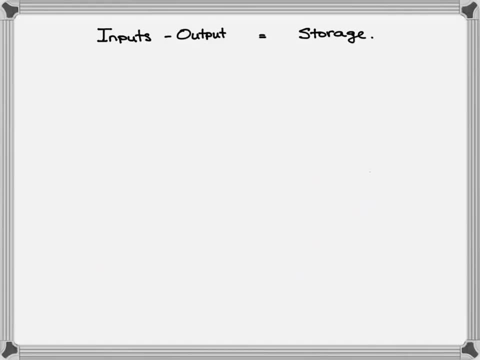 itself. As mentioned earlier, this could be a lake, a river, a roadway and so many other things. The governing equation for a hydrologic budget is the input minus the output equaling the storage. Both input and output are rates of water. A rate is something per unit time. In our case, we'll be dealing with depth of